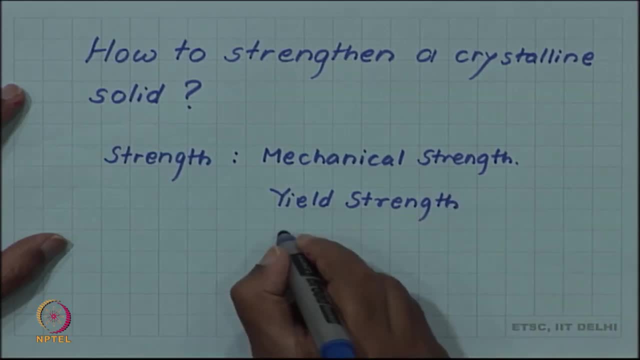 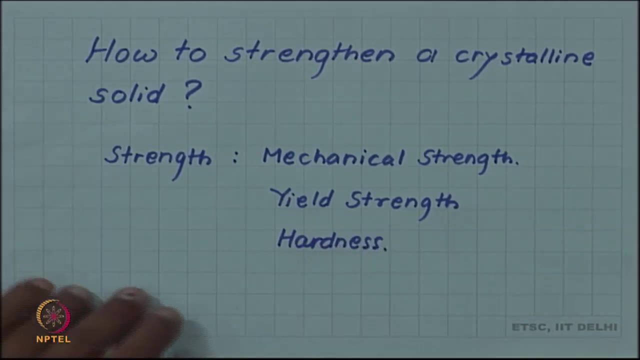 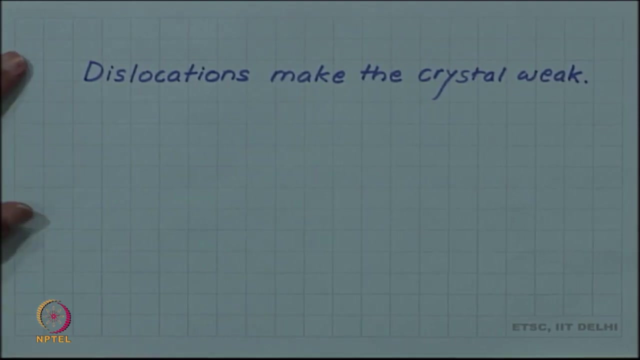 these are measures of mechanical strength and in many applications, higher the strength, better it is, because it can carry more load, or it can be used for reduction of the weight because a smaller cross section of the material can carry the desired load. So how to strengthen materials? Now? what we have been discussing, now that dislocations, 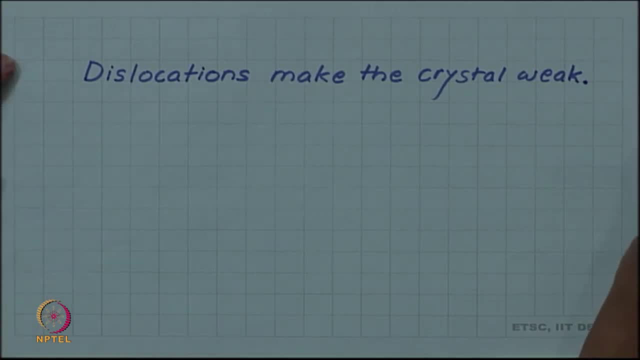 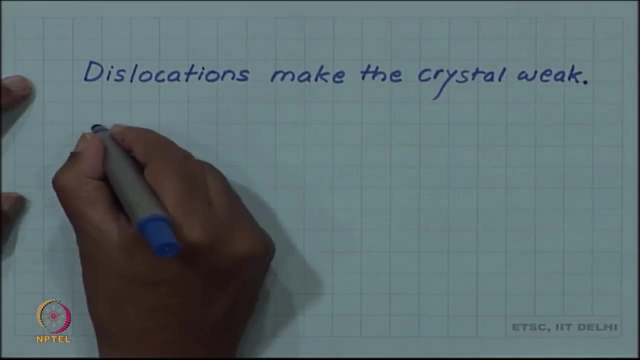 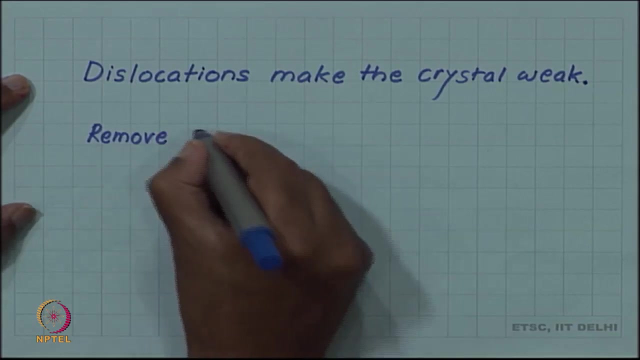 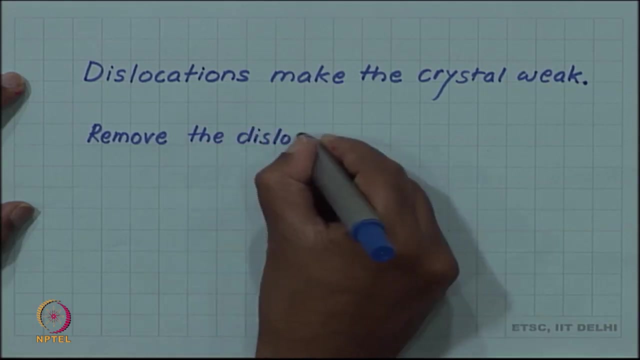 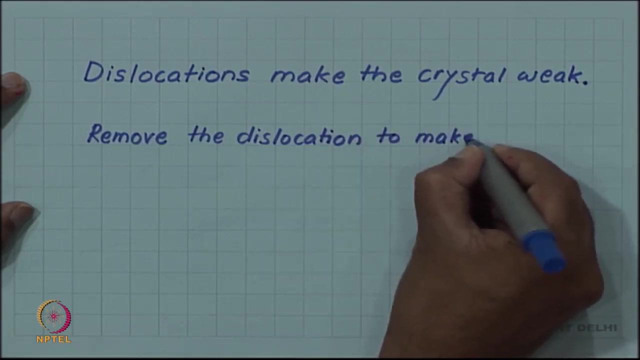 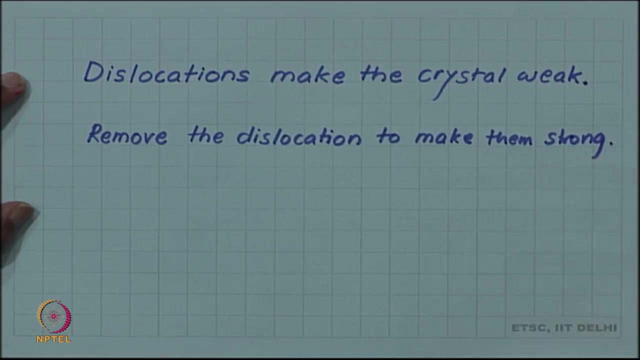 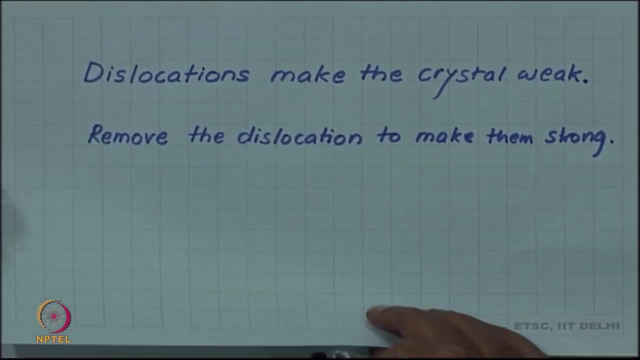 make the crystal weak. This was the content of the last video. So one can think of a way of strengthening as simply to remove this dislocations. Remove the dislocations to make them strong. only, this is not a very practical suggestion because in most cases 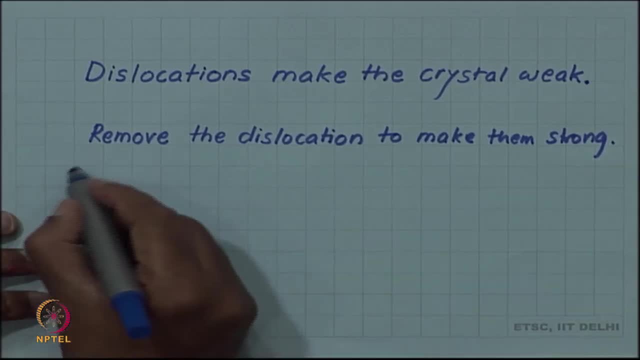 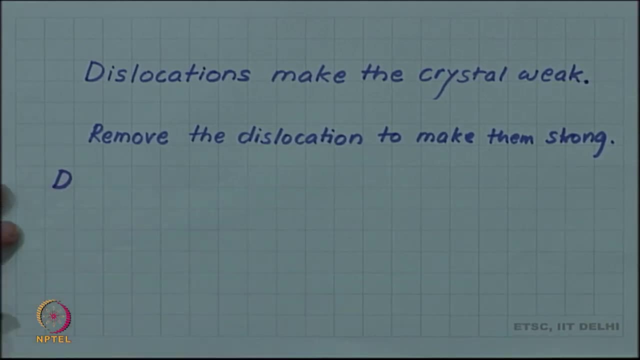 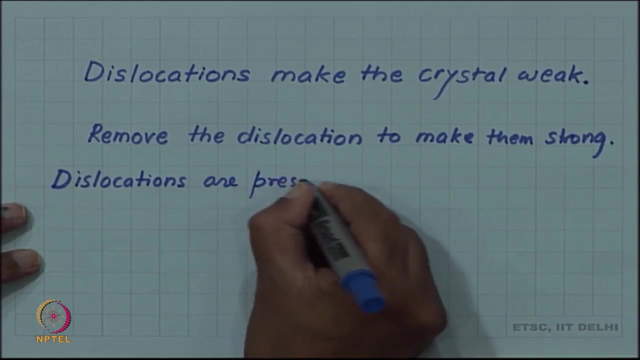 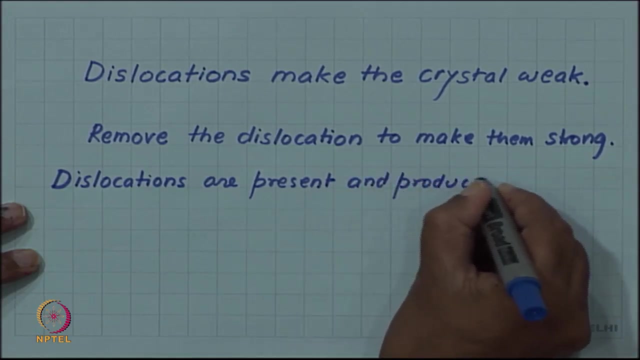 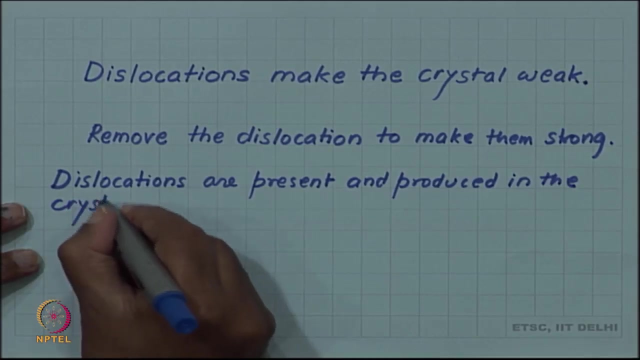 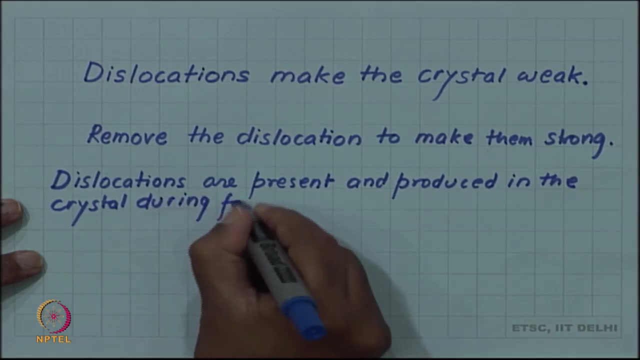 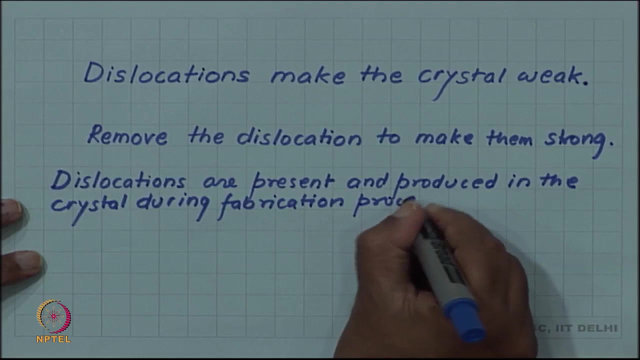 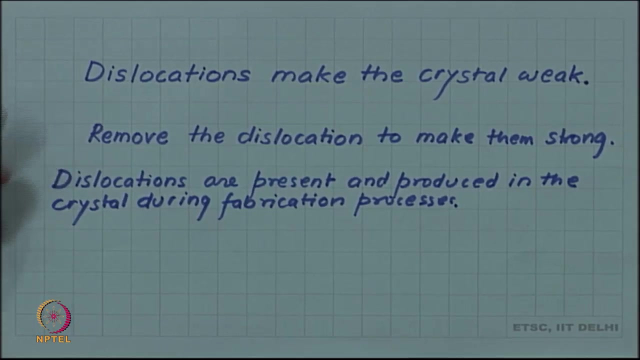 The dislocations actually appear in the crystal during production and fabrication processes. So dislocations are naturally present in the crystal and they are produced in the crystal during fabrication processes. So this suggestion is not very practical because you cannot really make a dislocation free crystal making. 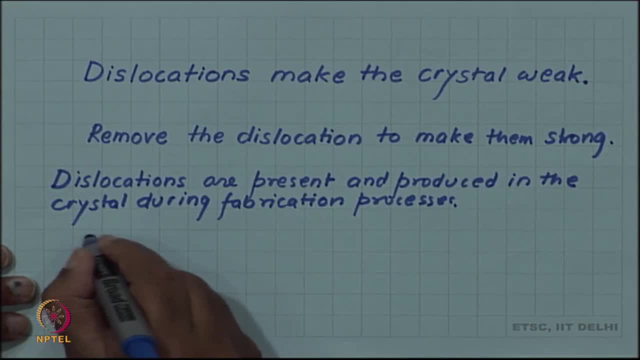 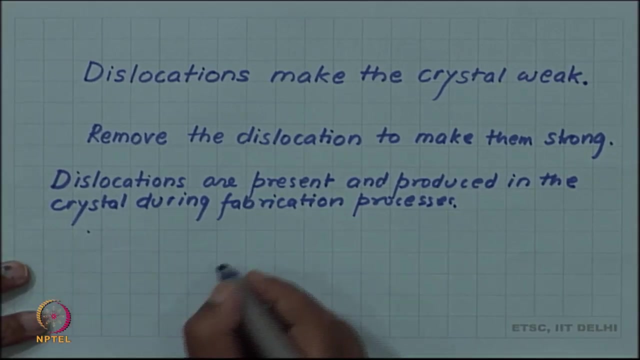 dislocation free crystal is not easy. Careful experimental control can sometimes produce dislocation free crystal, but that is done on a laboratory scale and in a smaller crystals and it is not very practical. So remove the dislocation is not a practical suggestion.